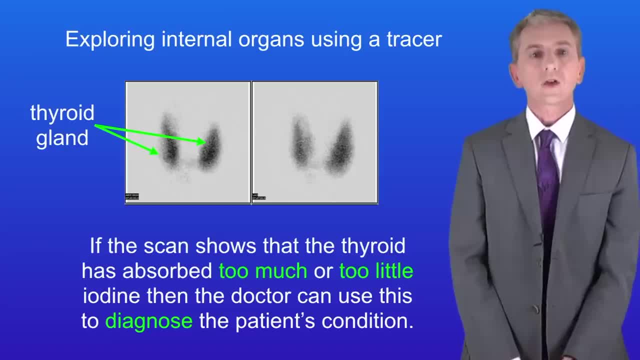 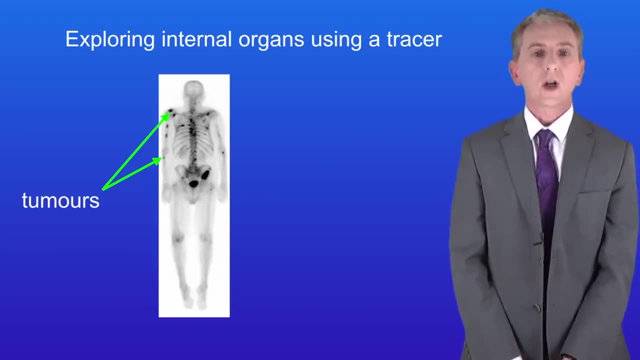 passes out of the body and can be detected. If the scan shows that the thyroid has absorbed too much or too little iodine, then the doctor can use this to diagnose the patient's condition. This shows a bone scan using a different type of radioactive isotope. Again, this one emits gamma. 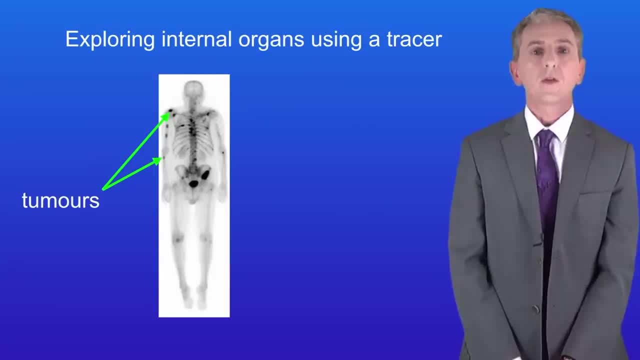 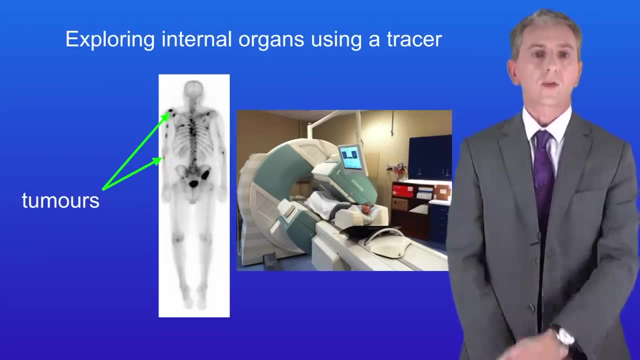 radiation Bone scans such as this one can be used to visualize damage caused by arthritis or to detect a problem with the thyroid gland. The second use is to explore internal organs and to detect tumors. This shows a person undergoing a bone scan using a radioactive tracer. 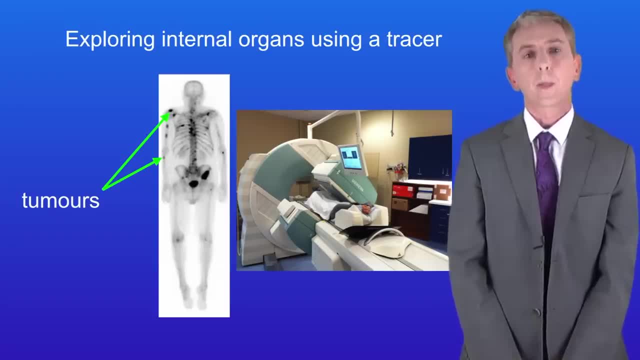 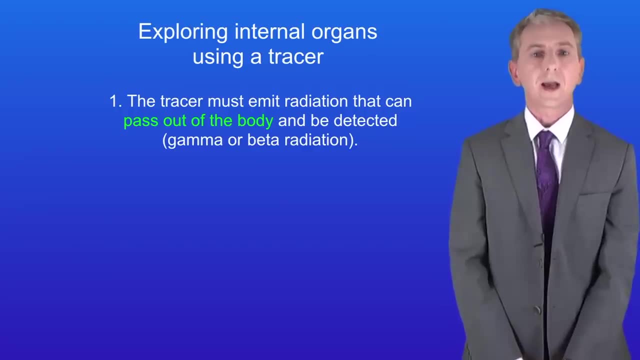 Now there are several issues to consider when using a radioactive tracer. Firstly, the tracer must emit radiation that can pass out of the body and be detected. So usually tracers emit gamma or beta radiation. Alpha emitters are not used as tracers, as alpha. 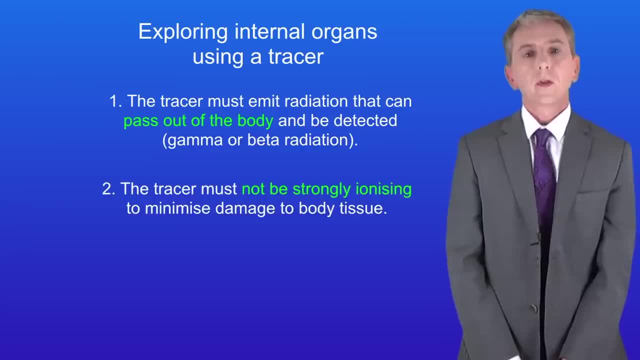 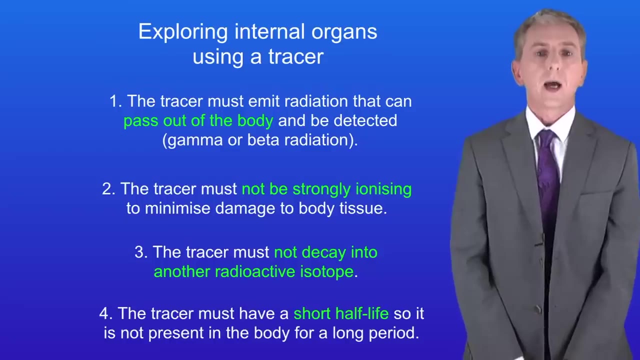 particles would not pass out of the body. The tracer must not be strongly ionizing to minimize damage to body tissue. Again, this makes gamma emitters good tracers. The tracer must not decay into another radioactive isotope And finally, the tracer must have a short half life. Now some 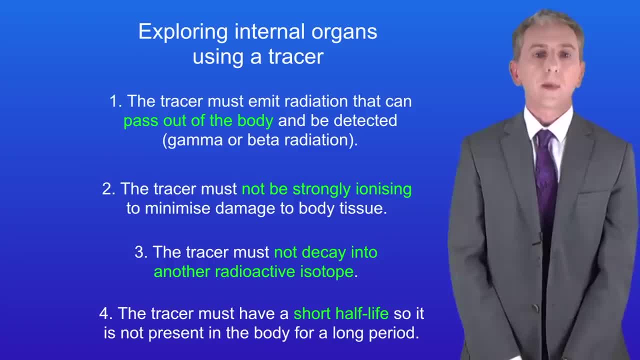 radioactive isotopes have got very long half lives and these do not make good tracers. That's because they continue to decay in the body for a long time and they can cause significant damage to body tissues. Radioactive isotopes have got other uses in medicine. 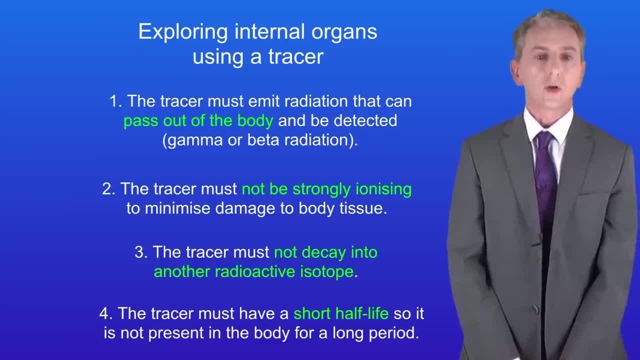 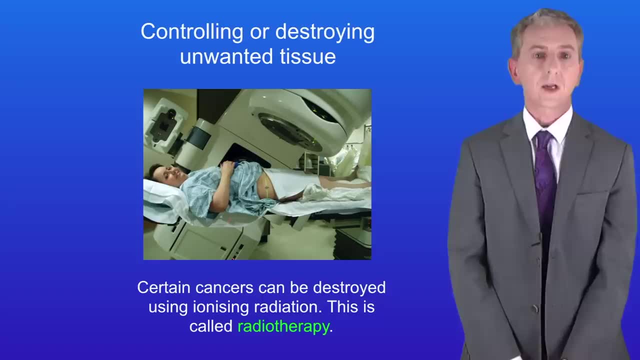 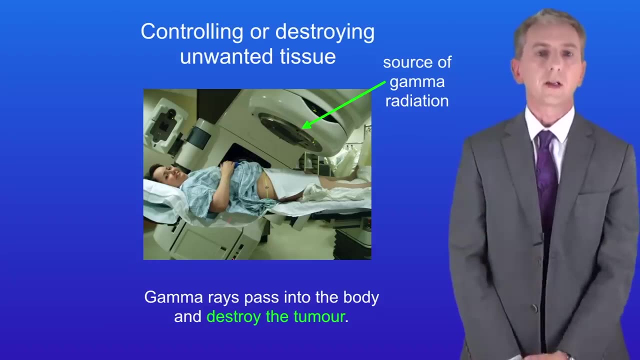 and one of these is to control or destroy unwanted tissue. So let's look at that now. A long time ago, scientists discovered that certain cancers can be destroyed using ionizing radiation, and this is called radiotherapy. I'm showing you here a patient undergoing radiotherapy. 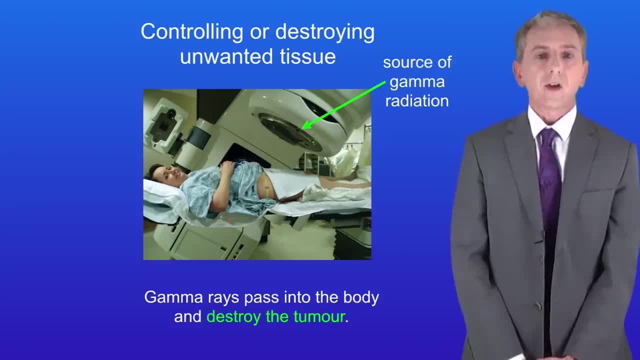 The machine contains a source of gamma radiation. The gamma rays pass into the body and destroy the tumor. One of the problems with this type of treatment is that healthy tissue may also be damaged as the radiation passes through the body. Now, in the case of this patient, 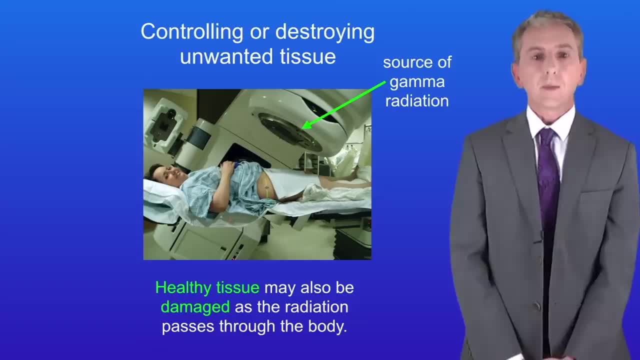 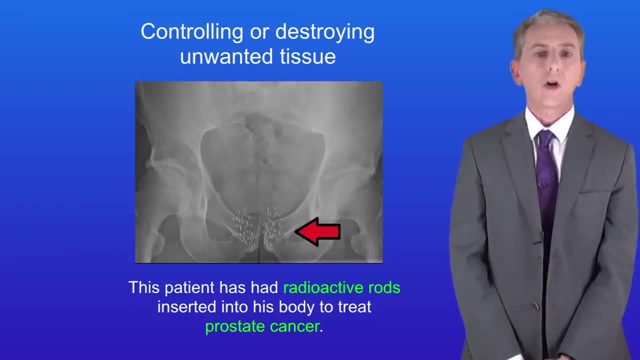 the radiation source is outside the body. but there are treatments where the radiation source is placed inside the body. I'm showing you here a patient who's had radioactive rods inserted into his body to treat prostate cancer. The benefit of this is that the radiation